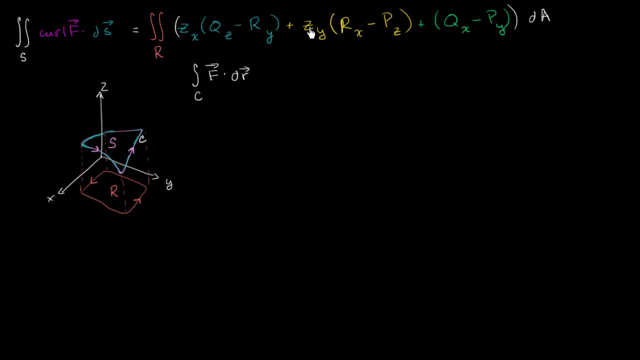 What we're going to see is that we're going to get the exact same result as we have right up here. But before we do that, I'm going to take a little bit of a detour to kind of build up to this. So let's just take this and put it to the side for now. 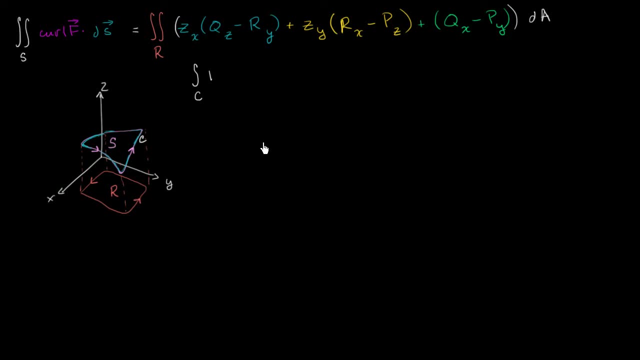 Let me actually just delete it right now, And what I'm actually going to do is I'm going to focus on this region down here, this region in the xy plane, And in particular. so this is path c, which is the boundary of our surface. 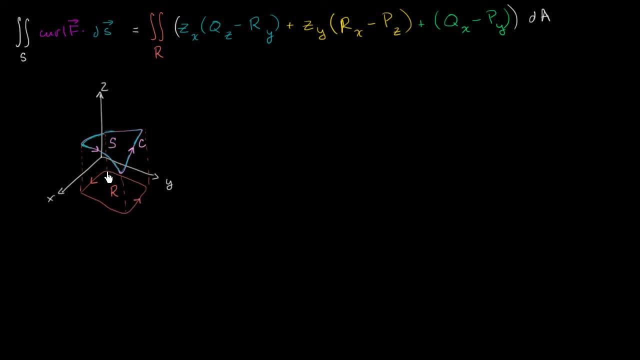 I'm going to focus on the path that is the boundary of this region, this path that sits in the xy plane, And I will call that path c1. And so one we can think about a parameterization of just that path in the xy plane. 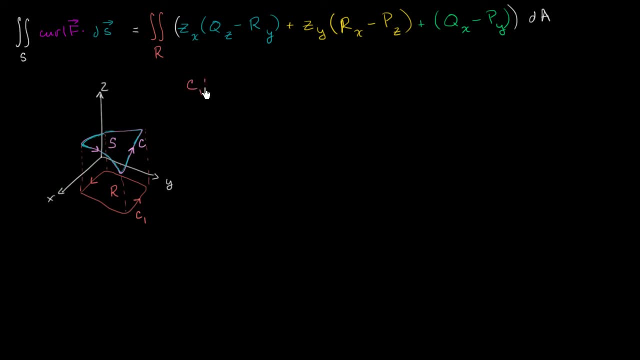 We could say that c1 could be parameterized as: x is equal to x of t and y is also a function of t And t is obviously our parameter and it can go between a and b. So maybe when t is equal to a it sits right here. 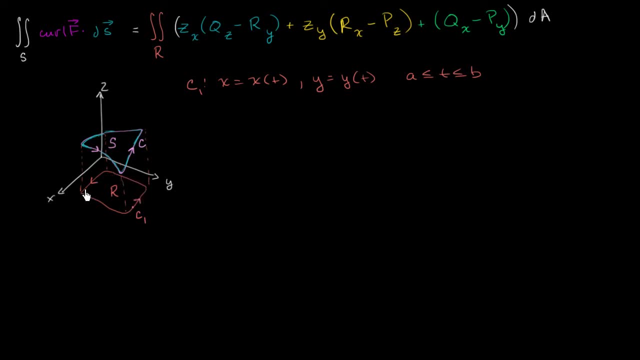 And then as t gets larger and larger and larger, it goes all the way around And eventually, when t is equal to b, it gets to that exact same point. So that's our parameterization, Right there. And now, just to make the rest of this proof a little bit more understandable. 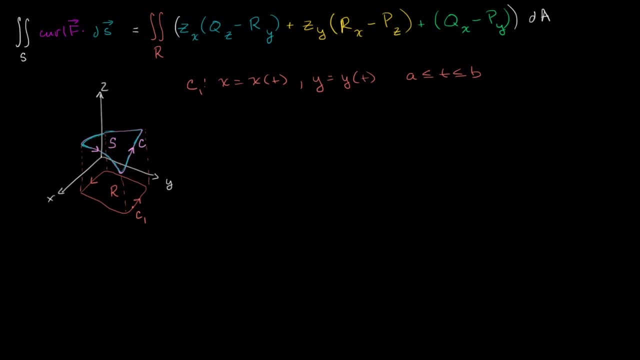 I'm going to give you a little bit of a review of something. Imagine that we have some vector field g, And g at minimum is defined on the xy plane So, and it could be defined other places. but let's say that g is equal to m of xyi plus n of xyn of xyj. 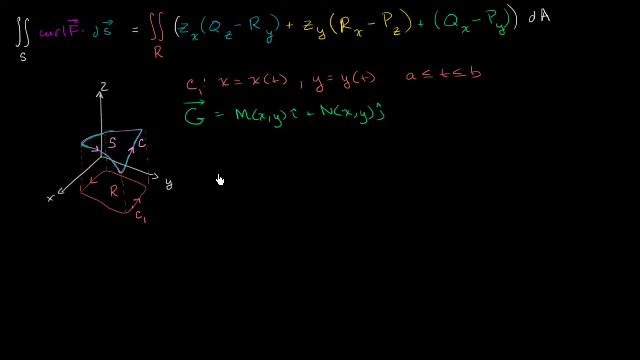 Now, what would the line integral- and this is all a review, We've seen this a long time ago- What would be the line integral over the path c1?? Not c, but this path that sits in the xy plane? What would be the line integral over the path c1?? 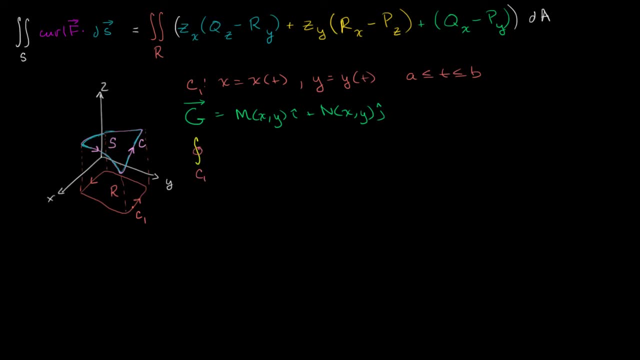 And I'll even- I like to write that sometimes Of, and I'm using g so I don't get confused with f, our original vector field Of g, of g, our vector field here along that path, g dot dr. 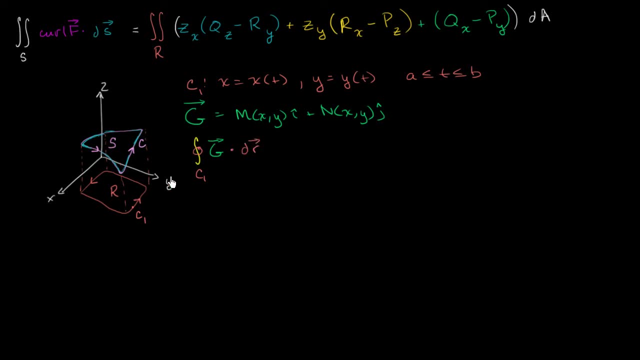 g, dot, dr. Well, dr, dr is just going to be equal to dx, dxi, dxi plus dy, dyj. So if you take the dot product of these two things right over here, you're going to get- you're going to get- the line integral over our path c1.. 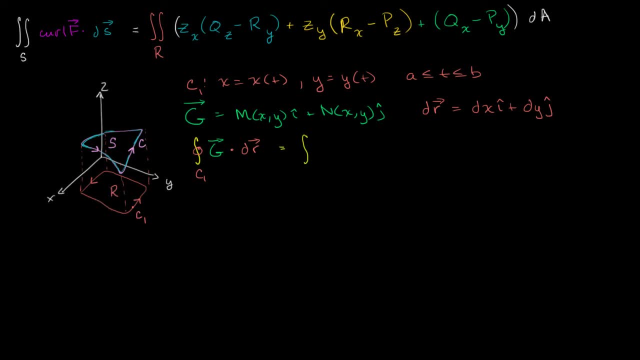 Remember, c1 is this path down here. Let me do it in that same color so you don't think I'm changing colors on you. The line integral over our path c1.. But when you take this dot product you have the. you multiply the x components. 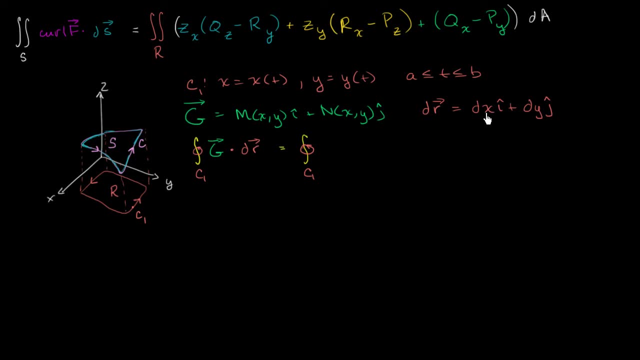 you add that to the product of the y components, So you have m times dx, you have m times dx, m times dx plus plus n times dy, n times dy. I just took the dot product of g and dr n times dy. 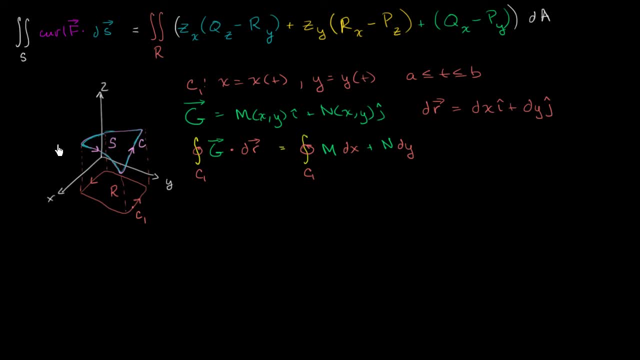 And when you evaluate these things, the one way to think about it is that dx is the same thing as- let me write it up here in a different color: And dx is the same thing as dx, the derivative of x with respect to t, dt, and same logic for y. 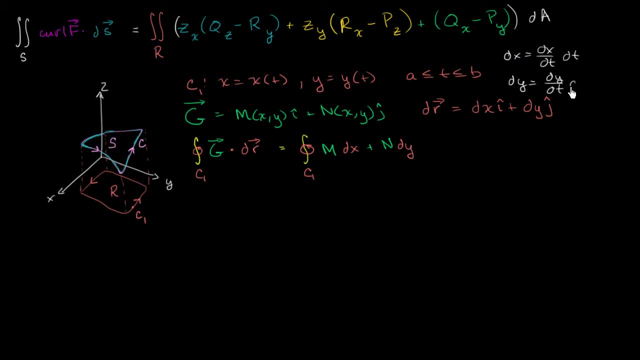 dy is equal to the derivative of y. with respect to t, dt, One way to think about it: these dt's cancel out and you are just left with dx, And this is an important thing to think about, because then this allows us to take this line integral into the domain of our parameter. 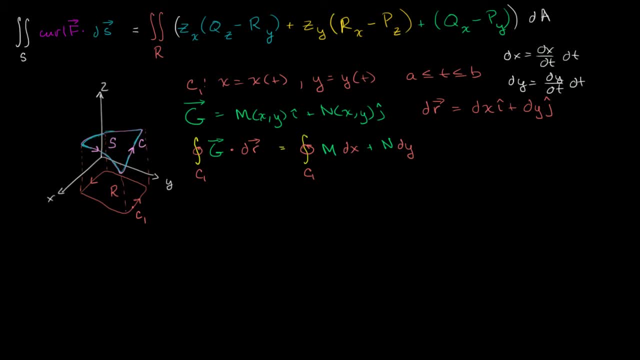 So then this will be equal to this, will be equal to this, will be equal to the integral in the domain of our parameter. So now we are in the t domain and t is going to vary between a and b. We are in the t domain, between a and b. 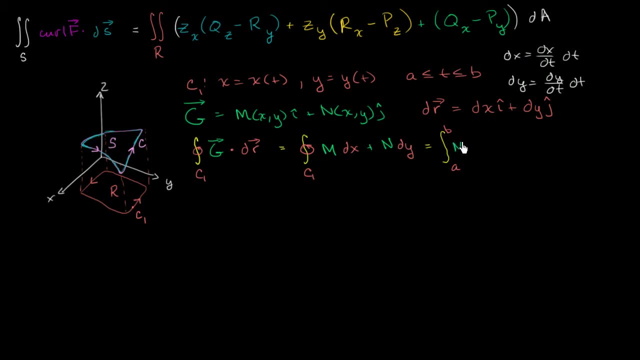 This is going to be equal to m m times. instead of writing dx, I'm going to write dx, dt, dt, So it's going to be dx. let me write it this way: dx, the derivative of x with respect to t. 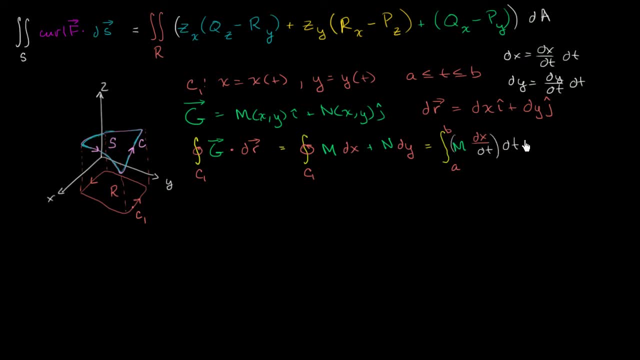 dt. that's the first expression plus plus n, and then the exact same thing: times dy, dt n, times dy, dt, n, times dy, dt, dt, dt. These are all equivalent statements. Now, with all of that out of the way, and this is really, 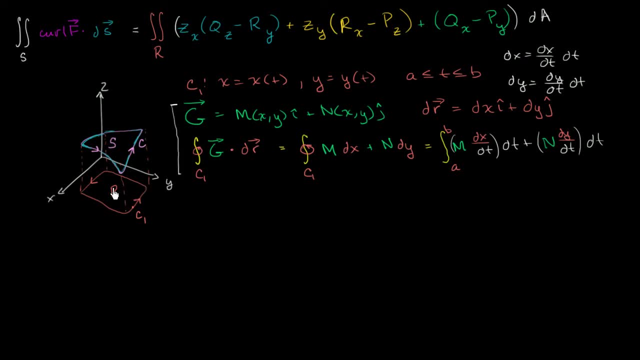 all of this is really just a reminder so that the rest of this proof becomes a little bit intuitive. With that out of the way, let's come up with a parameterization for this path up here for c, For c. Remember we just did c1 down in the xy plane. 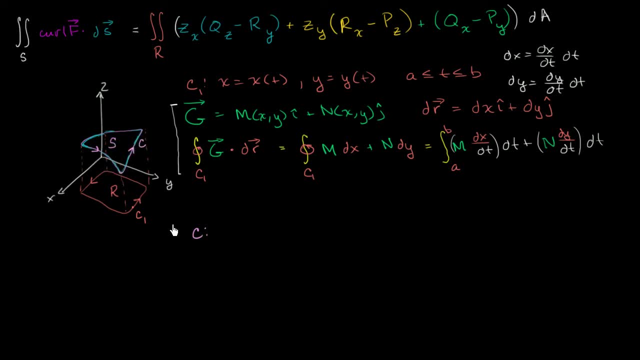 Now we're going to do c. that sits up here, that kind of rises above the xy plane. Well, for c, x can still be, the parameterizations for x and y can still be the exact same thing, because the x and y values. 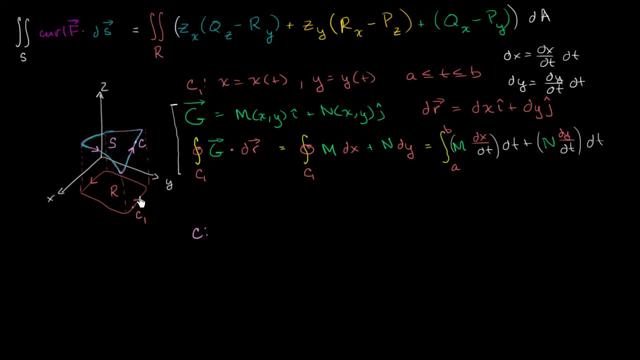 are going to be the exact same thing. The x value, the x and y value there is the exact same thing. It's the exact same thing as the x and y value there. The only difference is we now have a z component and we know we defined it way up here. 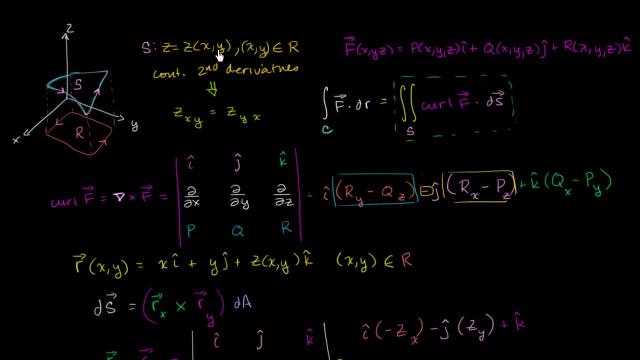 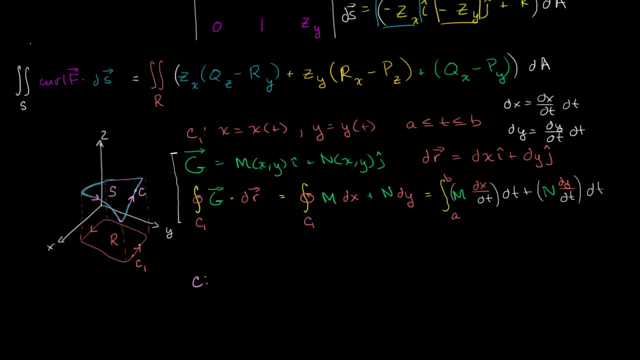 Our z component is going to be a function, is going to be a function of x and y. It tells us how high to go. So we can parameterize. we can parameterize c. as we can parameterize c, as maybe I'll write it as a vector. 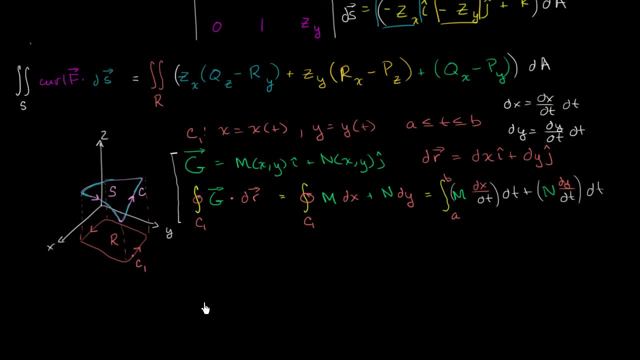 So let me write it, let me parameterize. So I'll write c as a vector C. Actually, no, I'll write it. let me write it this way. Let me write c. C can be written as. let me do that purple color. 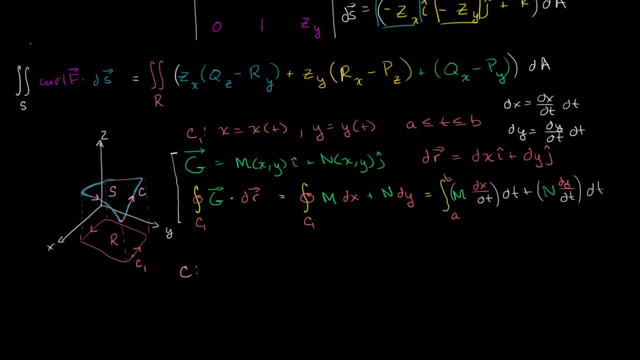 C we can say: is x, is x of t. Actually, let me write this as a vector. So I will write it and I'll use a vector r not to be confused with this r right over here. So these are two different r's, but I'll just use r's. 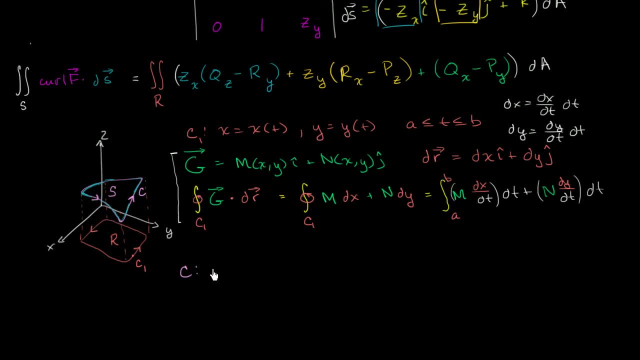 because that tends to be the convention. So in order to parameterize c, it's going to be the position vector r, which is going to be a function of t, And x is still just going to be x, x of t, i plus y of t- j.